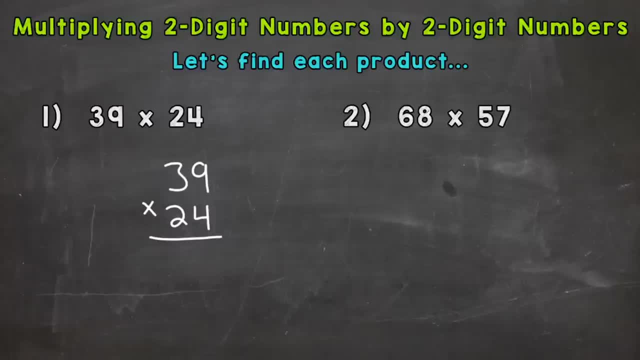 So let's go through this process, And the first thing we're going to do is 4 times 9,, which gives us 36.. Now we carry our 3 to the 10's place there. Next we do 4 times 30.. 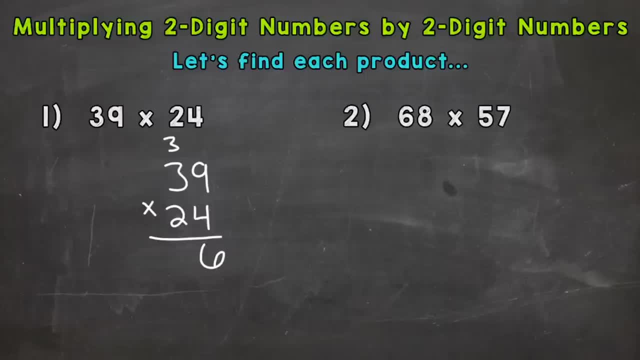 And I say 4 times 30 because the 3 and 39 has a value of 30. But we can just think of it as the simple digits of 4 times 3.. So 4 times 3 is 12, plus that 3 that we carried is 15.. 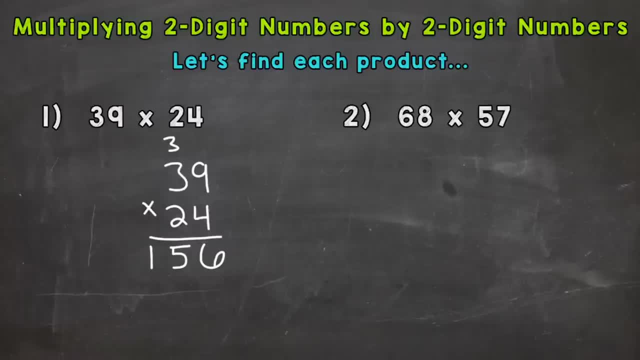 Now I'm just going to drop my 1 here because I don't have any more places to carry that 1 to. So I am done doing 4 times 39.. So I can cross off the 4 because I'm done with that. 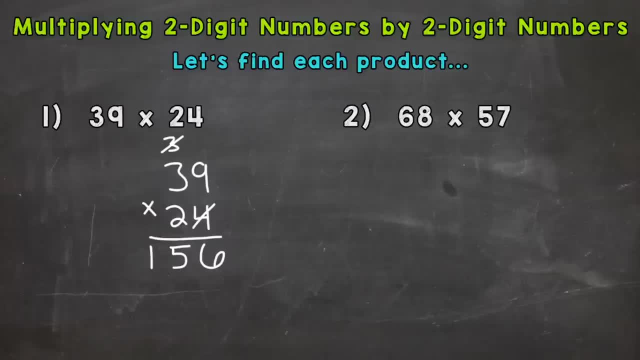 And I'm done with this 3 here. Crossing things off when you're done with it helps you so you don't get confused with any other numbers that we carry later on in the problem. Now this next problem we're going to do 4 times 39.. 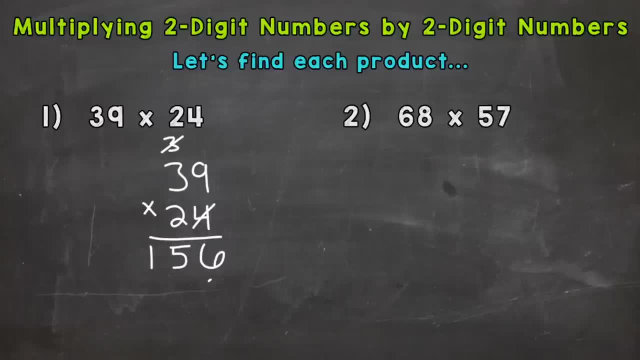 This next step is very important. We need to put a 0 here for when we do 20 times 39. And we put that 0 there because the 2 in 24 has a value of 20. So that 0 represents that. 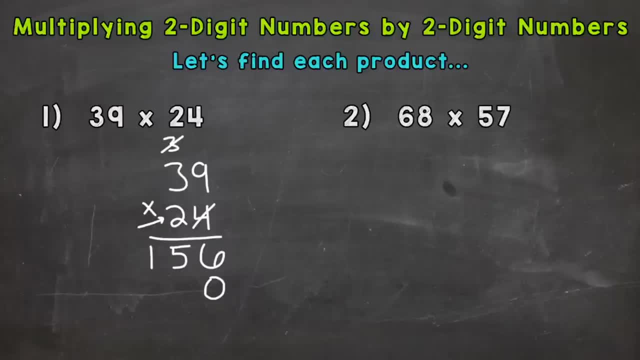 Now we go through our process. 2 times 9 is 18.. So we put our 8 and carry our 1.. See why we crossed out that 3 earlier, So we don't get it confused with any other numbers we carry. 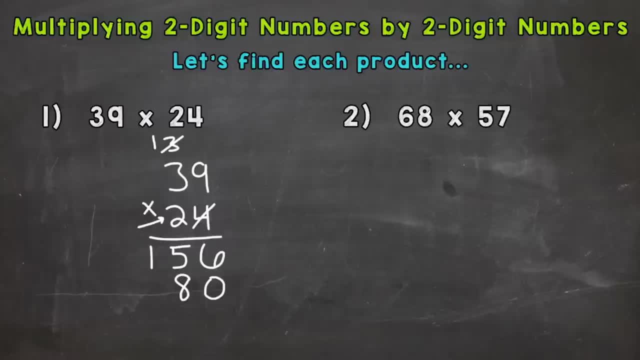 Then we do 2 times 3,, which is 6,, plus that 1 is 7.. So we have: 4 times 39 is 156, and 20 times 39 is 780.. Now we add these two answers together to get our final answer, or product. 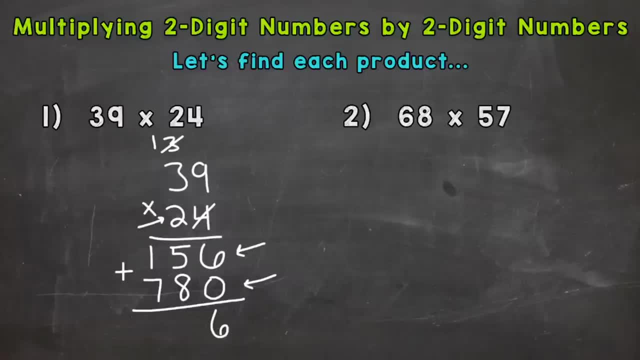 So 6 plus 0 is 6.. 5 plus 8 is 13.. 1 plus 1 is 2.. Plus that, 7 is 9.. So we get a final answer of 936.. So on to number 2, where we have 68 times 57.. 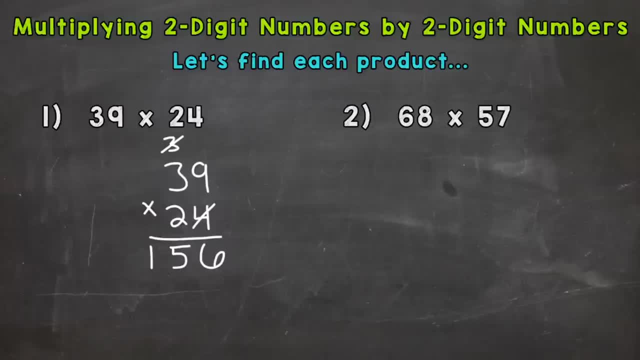 And I'm done with this 3 here. Crossing things off when you're done with it helps you so you don't get confused with any other numbers that we carry later on in the problem. Now this next problem is going to be 4 times 39.. 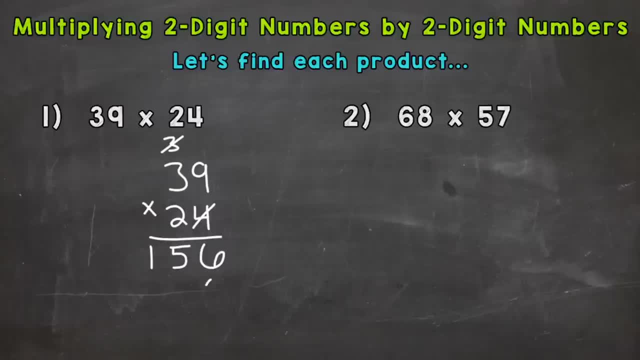 Now this next step is very important. We need to put a 0 here for when we do 20 times 39. And we put that 0 there because the 2 in 24 has a value of 20. So that 0 represents that. 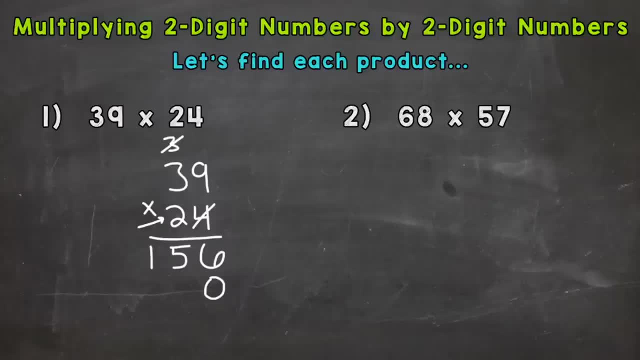 Now we go through our process. 2 times 9 is 18.. So we put our 8 and carry our 1.. See why we crossed out that 3 earlier, So we don't get it confused with any other numbers we carry. 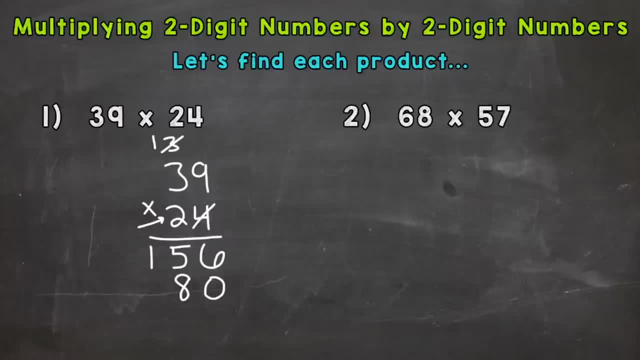 Then we do 2 times 3, which is 6.. Plus that 1 is 7.. So we have: 4 times 39 is 156.. And 20 times 39 is 780.. Now we add these two answers together to get our final answer, or product. 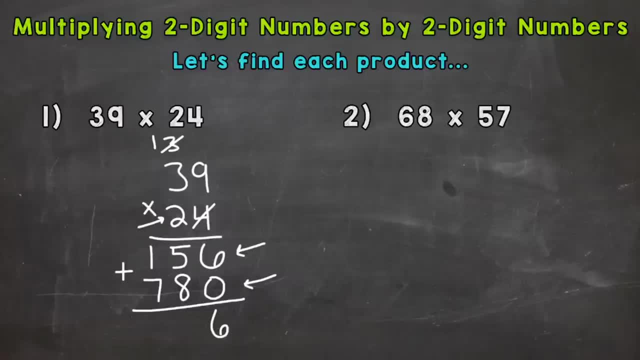 So 6 plus 0 is 6.. 5 plus 8 is 13.. 1 plus 1 is 2.. Plus that, 7 is 9.. So we get a final answer of 936.. So on to number 2, where we have 68 times 57.. 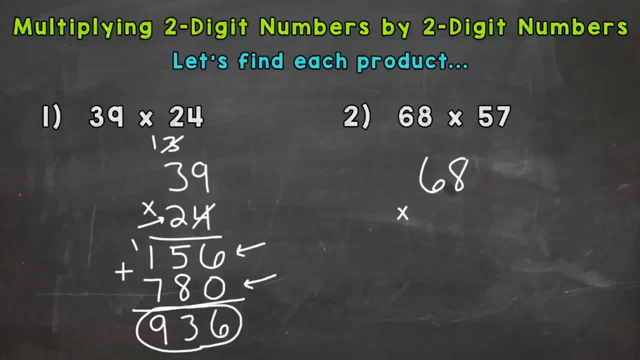 So let's line our problem up, And now we're ready to solve. So we need to do 7 times 68 and 50 times 68.. 7 times 8 is 56.. Carry our 5.. 7 times 6 is 42.. 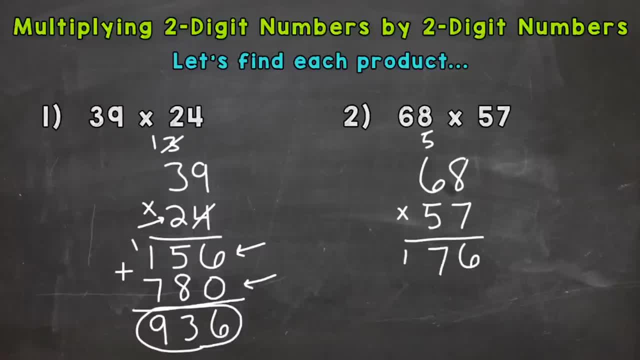 Plus 5 is 47.. So we get 476.. We are done with this 5 here And we are done with this 7.. Now that we're moving over to the 5 of 57.. That 5 has a value of 50.. 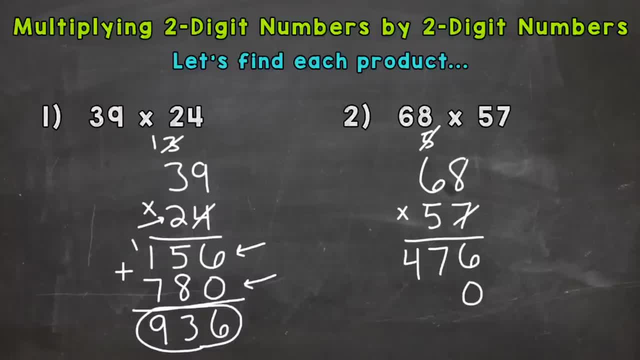 So we need a 0 here before we can continue on. Now we do 5 times 8, which is 40. So we have a 0.. Carry the 4.. 5 times 6 is 30. Plus that 4 is 34..